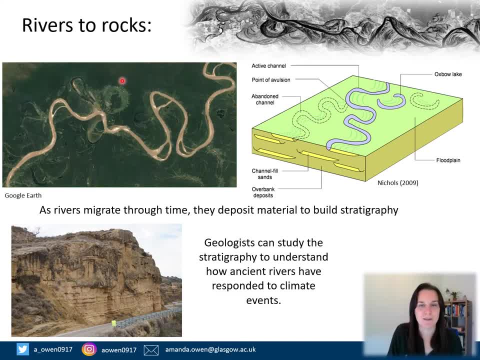 that previous channel. there We can also see another relic, one here. We're also going to get through time. that river flood and supply material to the floodplain. So what we end up with, as this diagram shows, is this river system migrating, depositing material, and then we have flood events, deposits in the mud and we build. 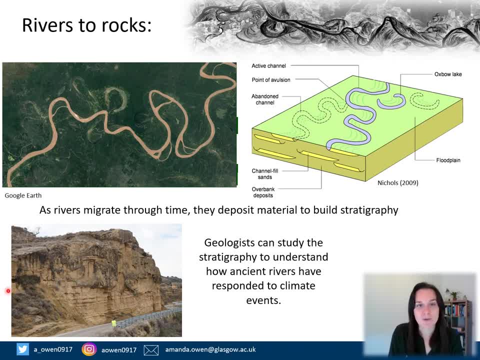 that stratigraphy through time. So what we can do is go and study the deposits of that stratigraphy in relation to climate events. Now we importantly have to identify where those climate events are. we will do in our case, study example. but we can then see and compare the river system. 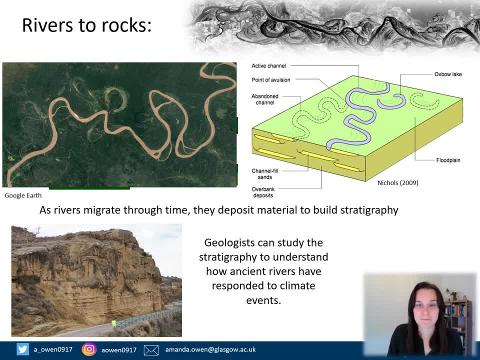 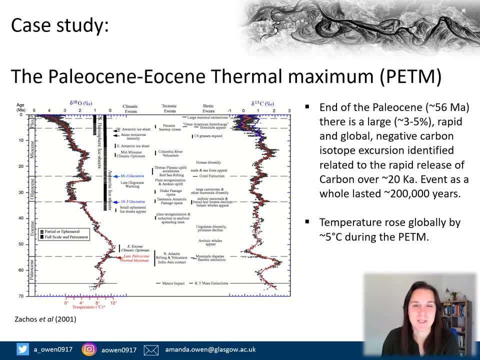 how it behaves before, during and after that event. So the Paleocene-Eocene Thermal Maximum records a pretty drastic climate event that happened about 56 million years ago. So just to kind of give you a little bit of context, we have on this graph we have age. 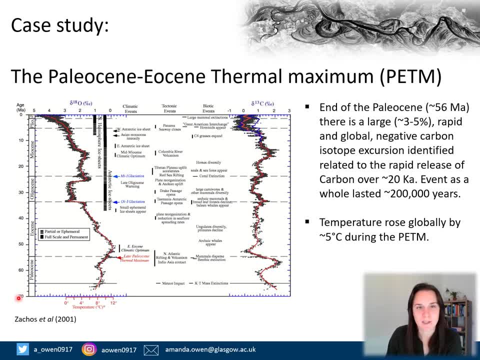 in millions of years: zero. so this is present day, down to 70 million years. There's a lot going on, but I'd just like you to concentrate on the temperature curve down here in red We can see from about the record we have here. we can see the temperature fluctuates through time. 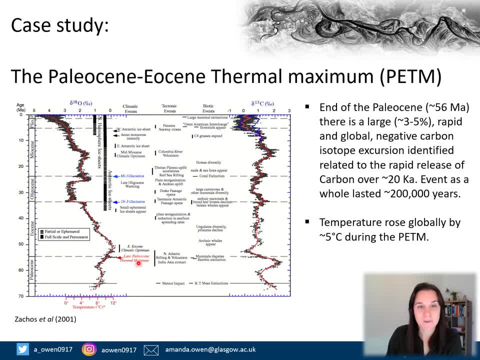 but importantly, we see a really drastic, sharp shift in the temperature through this negative carbon isotope curve about 56 million years ago, and this is because we had a really rapid release of carbon which took about 20,000 years to release On the whole the event, the Paleocene-Eocene. 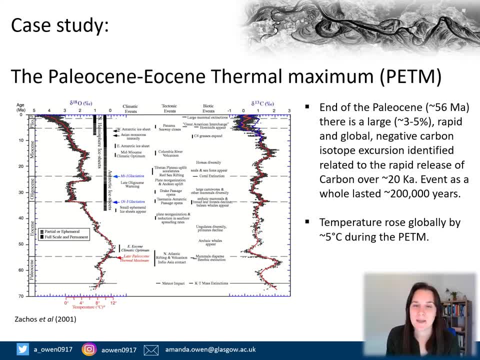 Thermal Maximum lasted about 200,000 years Now. globally, temperatures rose by about 5 degrees C during the Paleocene-Eocene Thermal Maximum. I'm just going to shorten that to PTM from now on so we don't get tongue-tied. So let's go and have a look at the Paleocene-Eocene Thermal Maximum. 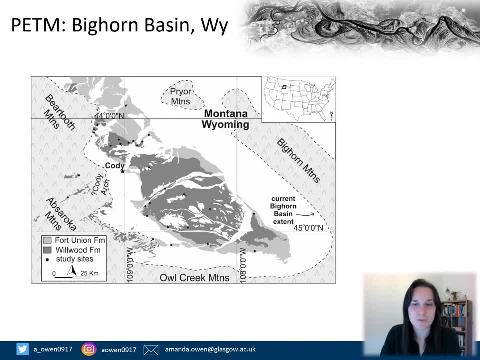 So the location we're going to go and have a case study example from is the Bighorn Basin, and this is situated on the border between Montana and Wyoming, so we're up in the northwestern corner of the USA Now. during the Paleocene-Eocene, so about 56 million years ago, we had collisional 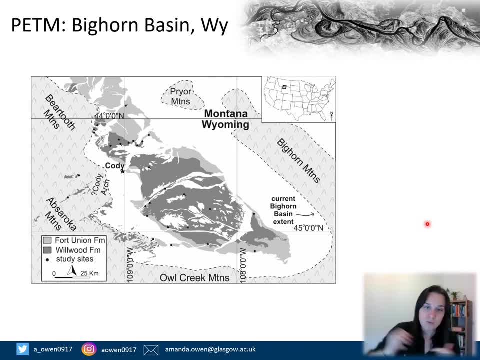 tectonics happening here, So we were having rocks being thrust on top of each other to form areas of uplift, and these areas are the Beartooth Mountains, the Owl Creek Mountains and the Big Horn Mountains over in the east. Now this is where we had areas of uplift and in between these we had 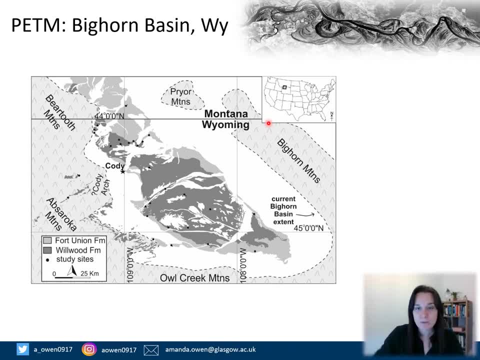 subsidence, so that's where our sedimentary basin is. So we had rivers coming from the Big Horn Mountains, from the Owl Creek Mountains and the Beartooth Mountains, delivering sediment into the center of that basin, and that's the sediment that we're going to go and analyse. 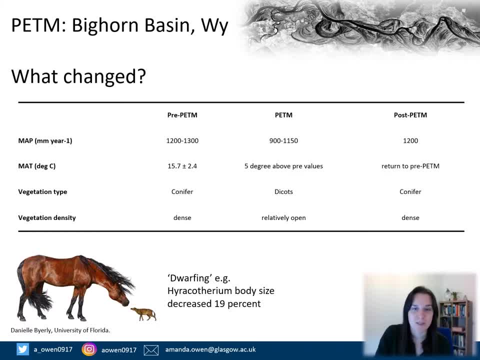 So what specifically changed in the Big Horn Basin during the PETM? So this table here summarises all the kind of literature that's been undertaken and studies undertaken in this basin. So we've got pre-PETM, PETM and post-PETM. 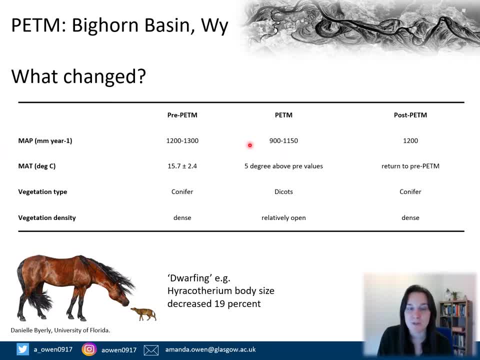 Now the mean annual precipitation. we can see that vastly decreases during the PETM and then recovers to normal conditions afterwards. The mean annual temperature we can see, like we saw globally we can see a five degree increase in temperature But again after the PETM it returns to normal conditions. 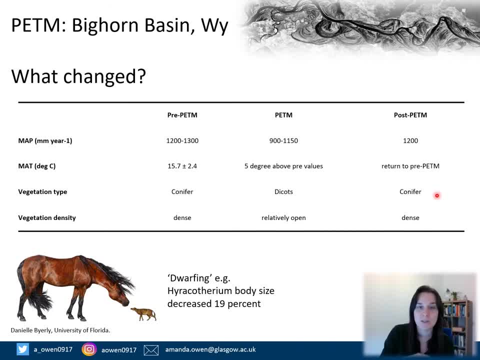 We also see a change in the vegetation type. so we go from conifers to dicots and then back to conifers. Also, the vegetation density changes. so we go from quite a dense mosaic landscape to relatively open vegetated landscape, but then again back to dense. 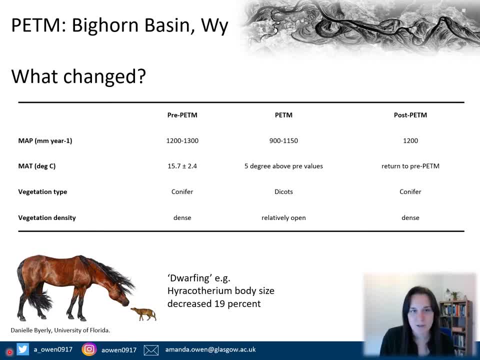 after the PETM. The other thing we see, which paleontologists have picked up on, is dwarfing of animals. So this is a sketch to show a modern horse and the expected size of horses during this time period. But we actually saw during the PETM that these horses dwarfed by about 19% in size. 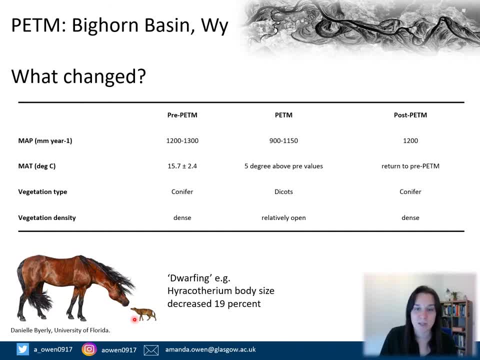 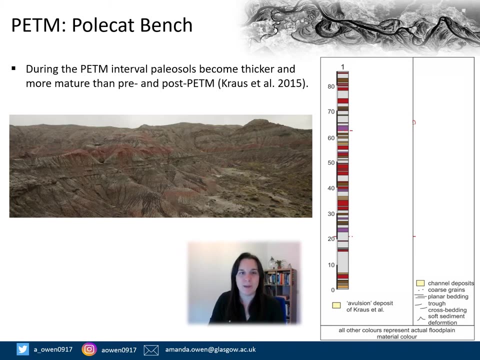 so there was a clear impact on the climate, on certain aspects of the environment. But what we're going to go and look at is how significant are these changes in terms of modifying our fluvial system, our river system behaviour? So the first site we're going to look at is a place called Polkat Bench. 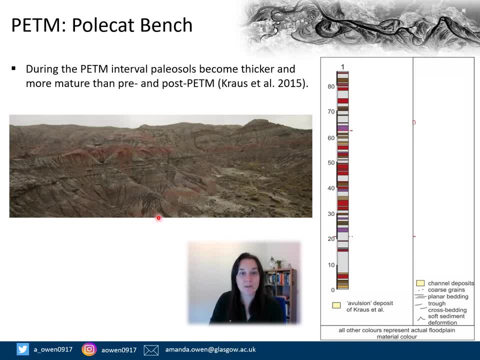 Scientists here have looked at the deposits and we have the carbon isotope here, so we know exactly where that climate event is. So we can look at the deposits before, during and after that event. Now we as sedimentologists create something called a sedimentary log and that basically means we go. 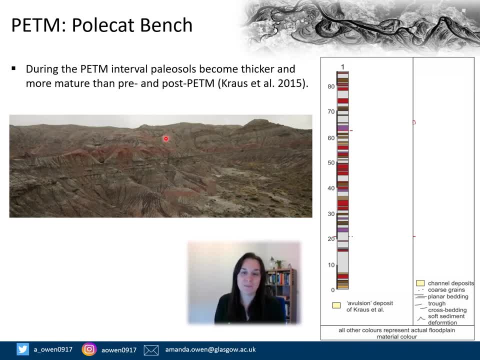 through a big piece of those layers of rocks and record information. So, for example, we record what the environment was, whether it was flood plain or river channels. We record important things like what's the grain size of the sediment, because that can tell us about the dynamics of the river system. 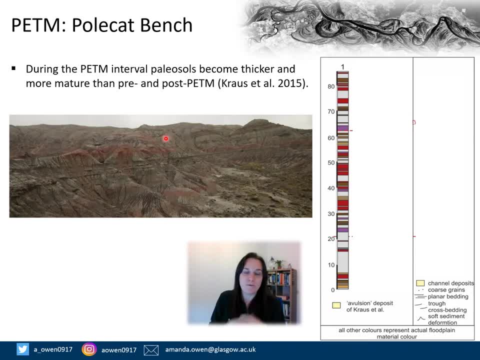 So, for example, larger grains are going to need much higher flow velocities than smaller grains. We can also record information, for example the colour of the rock, So we can see in here, even though it wasn't a particularly nice day that we went here. 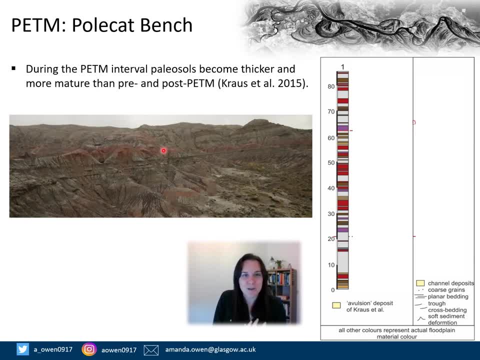 hence the grey photograph. but we can see some rocks are red and some are grey. So this is a very simplified sedimentary log here, and this red line here represents pre-PETM. this is the PETM info here and this is post-PETM. 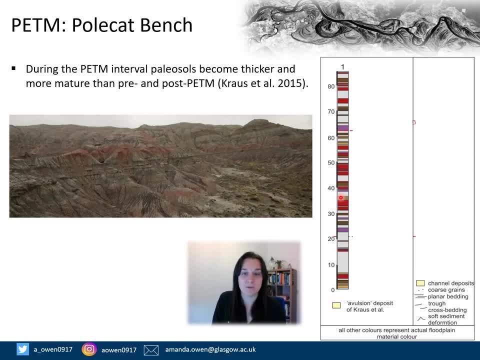 And the colours in here represent the colours of the paleosolids, which are basically ancient soil deposits. So we're looking at ancient flood plain. An important thing to understand about paleosolids is: just like modern soils, we have certain soils forming in certain 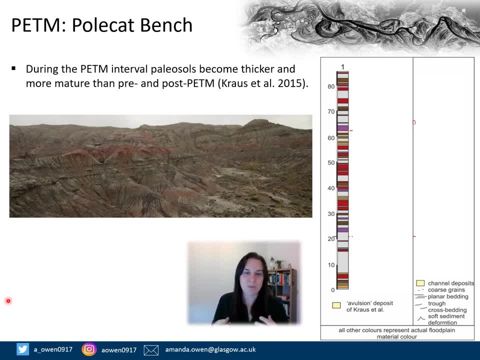 environments and certain climates. So grey soils represent very kind of waterlogged conditions, very wet, whereas red soils represent quite dry conditions where we have oxidation happening. That's what gives it that red colour. So I think we can all see at this site, here we have grey rocks, grey paleosols. 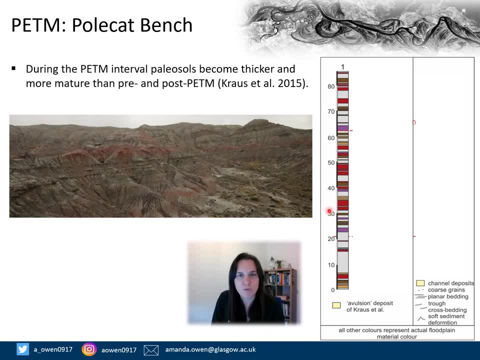 And then during the PETM the rocks become a bit more red And then again, although we still see some red rocks, we don't see that dominance of the red paleosolids after the PETM. That kind of indicates to us which researchers Mary Krause had done. 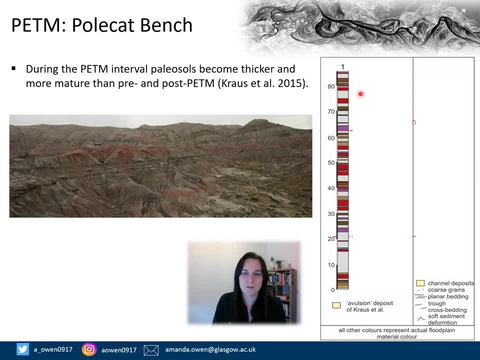 is that the soils became maturer and thicker and more red during that climate event, which matches with what we expect with the temperatures which we get from isotope data. However, there are certain things that don't quite add up here, So that sedimentary log- another one- was constructed hundreds of metres away. 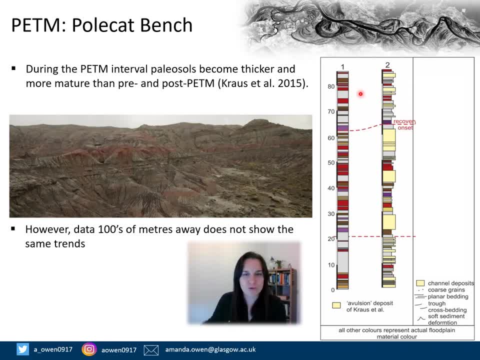 but we don't see the same trends, even if we just walk 100 metres away. And this is that sedimentary log here. So the yellow bit here that represents a river channel deposit. So we can see the difference here is: this is where the river was during the pine period. 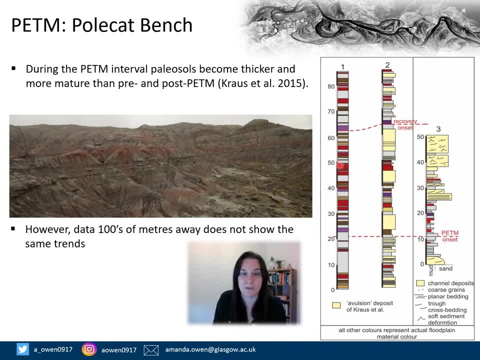 Over in this section that's just floodplain dominated, whereas over here we have a few river channels present And, yes, we do start to see those red deposits come through, but we can also see them before and after, So this log doesn't actually give us any indication. 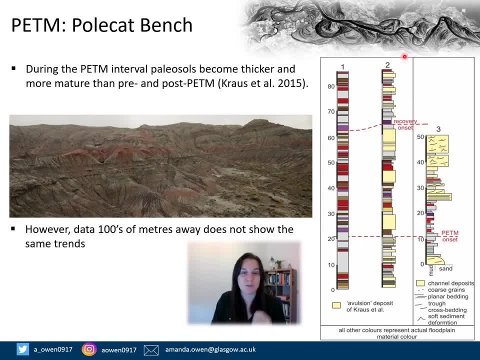 We do see channels present during that period, but we also see channels above and below it. We then constructed another sedimentary log ourselves, another few hundred metres away, And again we can see these river deposits as we go up through time through those layers of rocks. 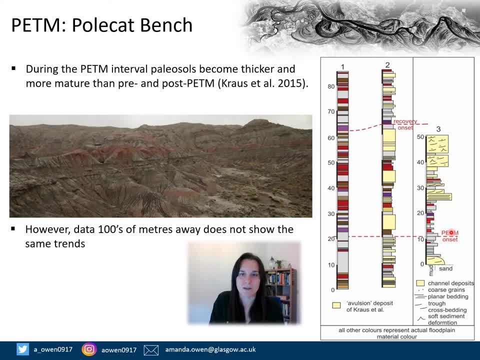 Again, we can see where the onset is because we have the geochemical, geochemical data, but again we're not seeing any kind of big, massive changes. And something that's really critical here is we only actually looked 20 metres below. 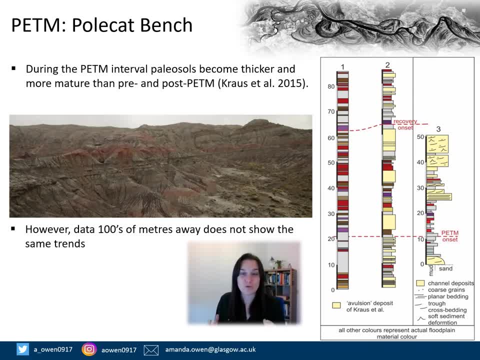 and about 20 metres above. In this basin we have hundreds of metres to kilometres of sediment. So that's the first thing that we kind of need to be careful of is, yes, we can look at the context of that PETM event. 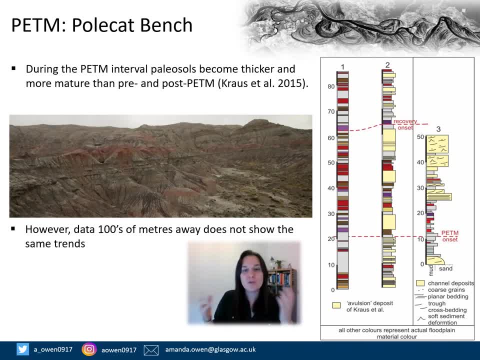 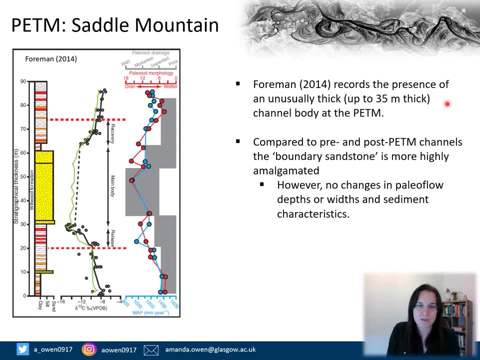 but how far above and below do we need to compare to understand what the normal conditions were? Then go over to Saddle Mountain, a new site, And a researcher here reports the presence of a really thick channel body here. so deposits of river channels on top of each other. 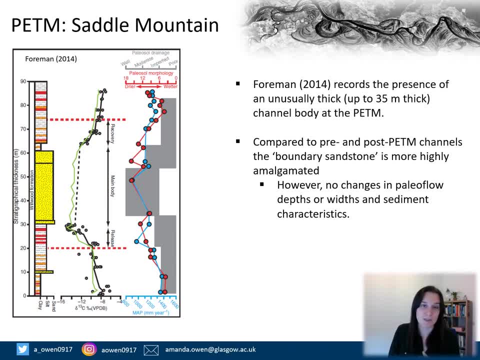 And they said it actually got to kind of record thickness: 35 metres thick. Now if you compare that deposit to pre- and post-PETM channels, the authors recognise that the PETM interval they had a much larger scale river system. 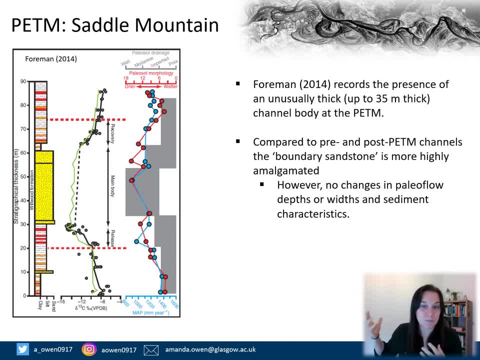 Now, if we think back to possibly at the previous site, that's where we actually saw the river floodplains become much more mature and much more kind of prevalent and thicker and hotter. So it is quite hard to explain how, in another area a few kilometres away, 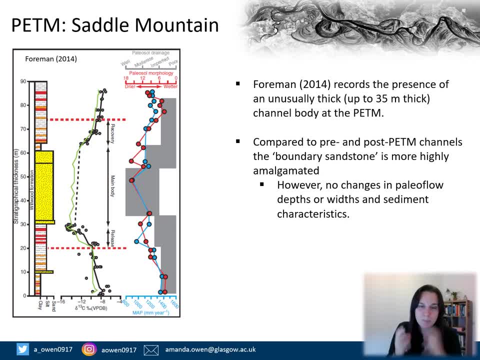 that we have this really big river channel come through. But an important thing is is, internally, the characteristics of the system didn't change, which the authors picked up. There was no change in the paleo flow depths. there was no change in the widths of the channels. 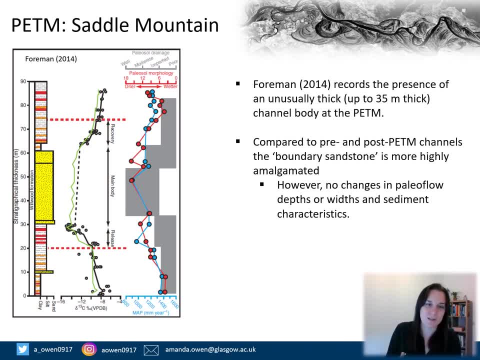 and there was no change in the sediment characteristics of, for example, grain size. So this again starts to make us think about: well, how much did that river change? All we have here is just more deposits on top of each other. 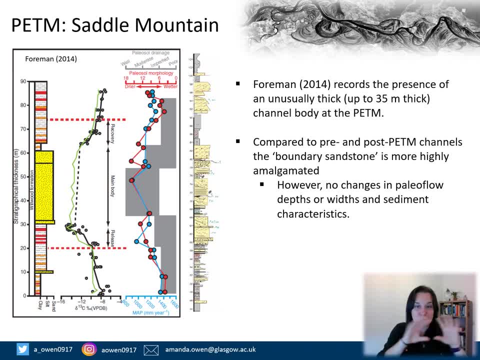 We also constructed a sedimentary log and we actually found that the river channel actually changes in thickness quite considerably. So this is a question is: where do you take your data point from? And this is the importance of doing these really large scale studies. 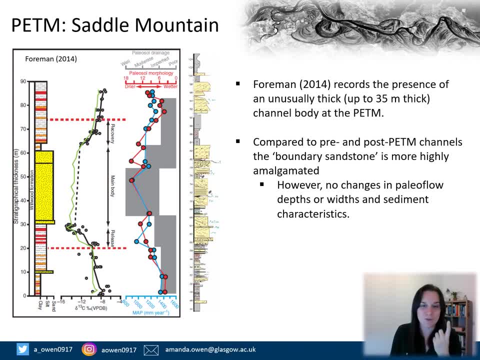 In that picture. we shouldn't ever base our interpretations on one data point. We should look at multiple data points and see what's happening. And this is actually demonstrated at the next site. very well, So at Sand Creek Divide, our final stop. 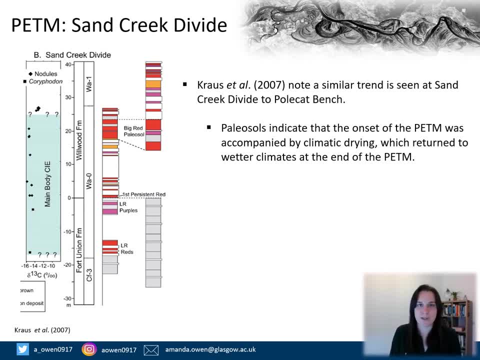 again, authors noted that there was a similar trend seen at Pole Cap Bench, where we have much more rather mature soils during this climate event which, in here, is just in there. However, the authors noted- and it's something that we noted with our data as well- 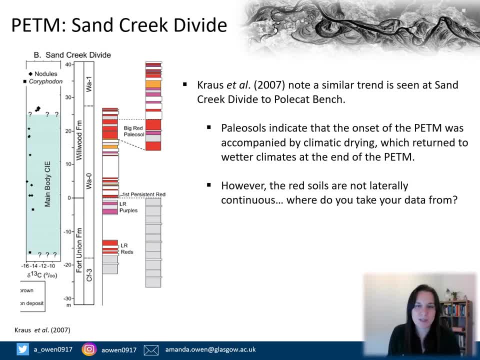 is, if you trace that red layer, those nice thick deposits, during that climate event, they actually change into grey deposits, even though we're in exactly the same time period. And this makes sense when you actually think about it, because if we stood on our modern landscape and we walk across a floodplain, 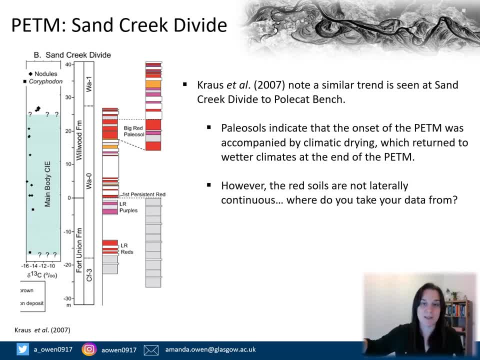 the dynamics and the characteristics of that floodplain change in space And that's exactly what's being recorded Here at these sites. we're not seeing the same changes happening all at once because our environment is extremely dynamic. We can walk from a river channel over onto very wet proximal, very close to the channel floodplain. 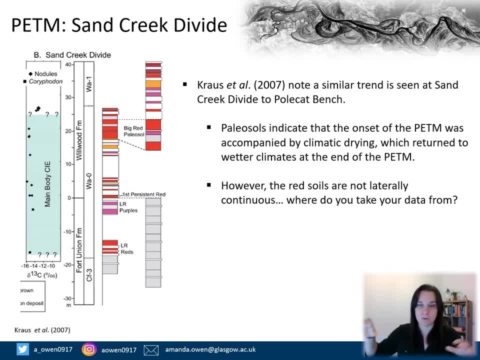 very distal, far away floodplain, And the characteristics of those environments change even in a snapshot. If we pause time and assess them, we're going to see those changes. So we need to understand at a very large scale with multiple data sets. 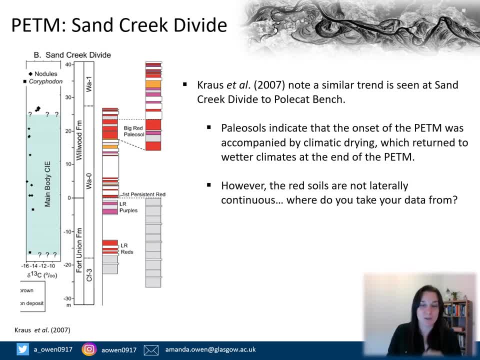 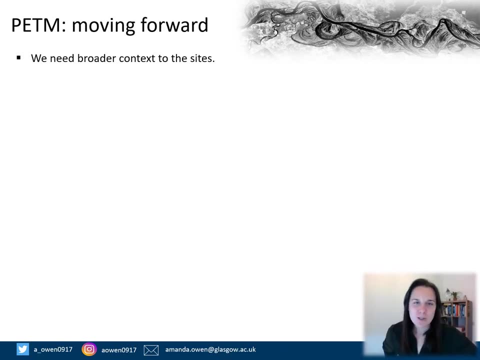 what is happening. And again, we need to consider what's happening at an appropriate depth, below and above, to make sure our comparison of what's happening at that climate event is true and we have proper context to it. So our work has shown that we do actually need broader context to the sites that we're studying. 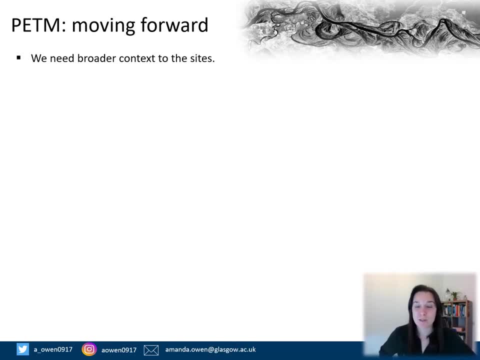 It's not enough to go and study one site because you're studying one point on the landscape. We can walk across our landscapes and see that it changes. so therefore, different parts of the landscape We would expect should respond differently to the event. So what we're doing is studying multiple sites across the basin. 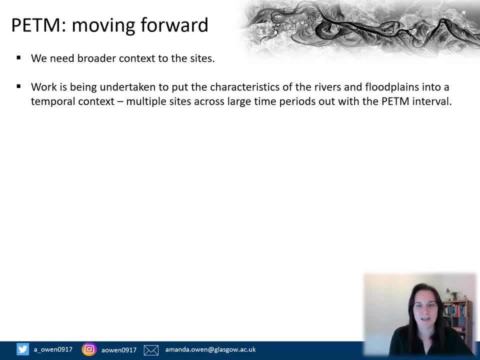 to ensure that we gain that good spatial understanding of any possible changes. We're also significantly increasing the amount of sediment we compare the climate event with. So we've got about 4000 metres of sediment now analysed to make sure that we have true context as to what happened before and after the event. 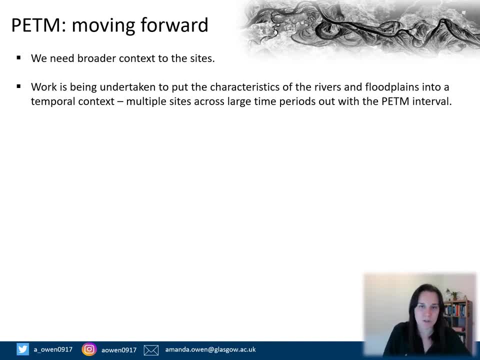 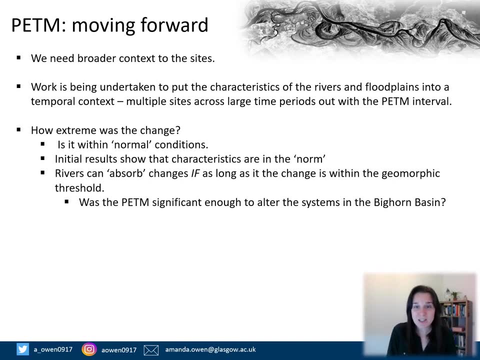 to see how significantly different the climate event was in some of the river characteristics. So how extreme was the change? Well, hot off the press is actually the river characteristics within the normal range of what we saw before and after the climate event. So this actually implies to us that the river didn't see any significant changes. 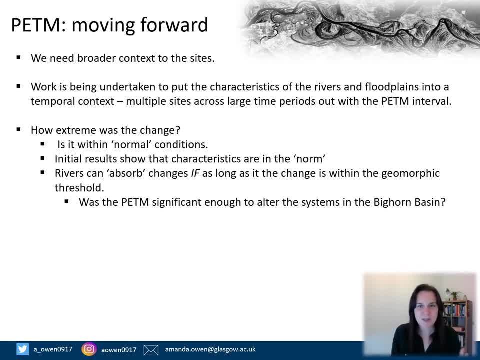 as a result of that increase in climate. So does that mean that there's nothing to worry about? Well, actually no, and for reasons I'll explain now. Rivers can absorb changes. They can kind of they go through kind of a self-organisation process. 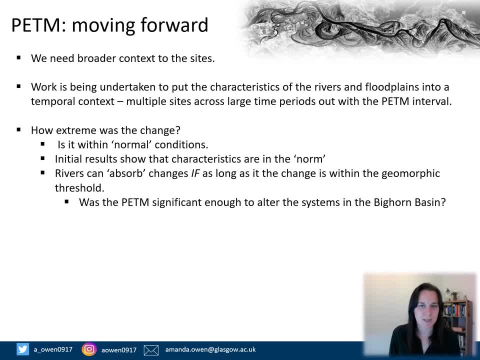 They can kind of absorb any changes that are coming in, But only to a certain extent can they do that And we call this the geomorphic threshold. So if the change is too great, we go over a geomorphic threshold and we see significant changes in the river behaviour and the characteristics. 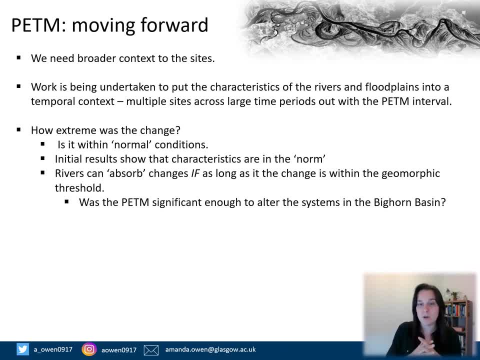 So we believe for this climate event that actually the change was over a long enough time period for the river to kind of absorb those changes. But this is a clear work in progress And what we're trying to do at the moment is to do some modelling to see using our data set.